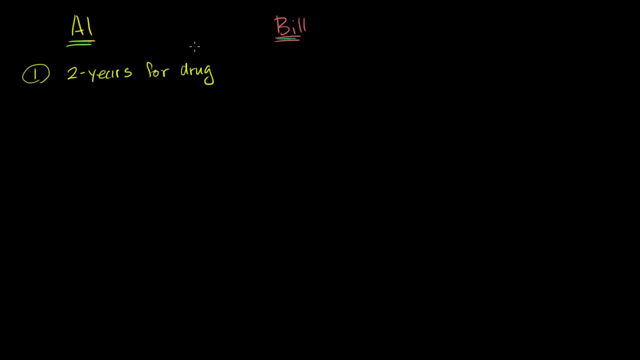 is his hunch, his suspicion. He has no hard evidence. So what he wants to do is try to get a deal with each of these guys so that they have an incentive to essentially snitch on each other. So what he tells each of them is: look. 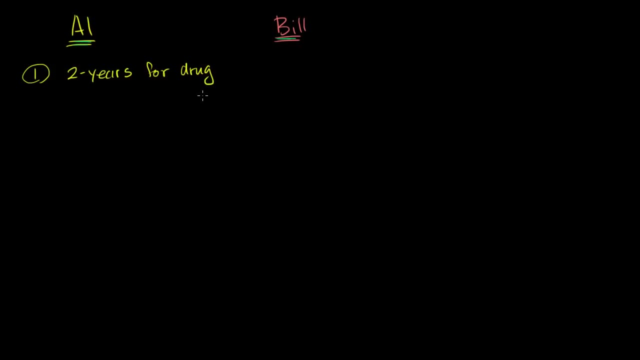 you're going to get two years for drug dealing. That's kind of guaranteed. But he says, look, if you confess and the other doesn't, then you will get one year And the other guy will get 10 years. So he's telling Al: look, we caught. 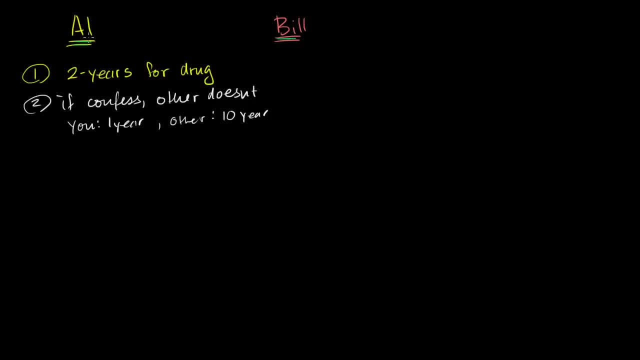 Bill too, just randomly today, If you confess that it was you and Bill who performed that armed robbery, your term is actually going to go down from two years to one year, But Bill is obviously going to have to spend a lot more time in jail. 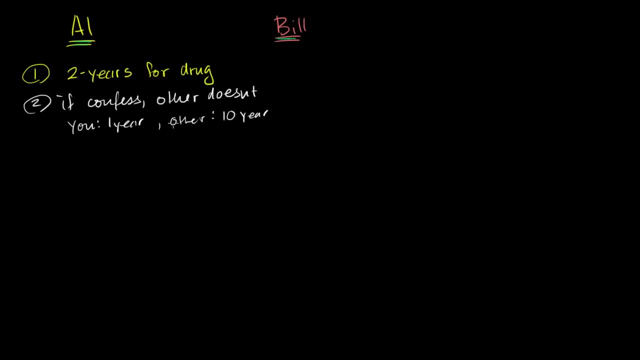 especially because he is not cooperating with us. He is not confessing. But then the other statement is also true: If you deny and the other confesses, now it switches around: You will get 10 years because you're not cooperating And the other your co-conspirator. 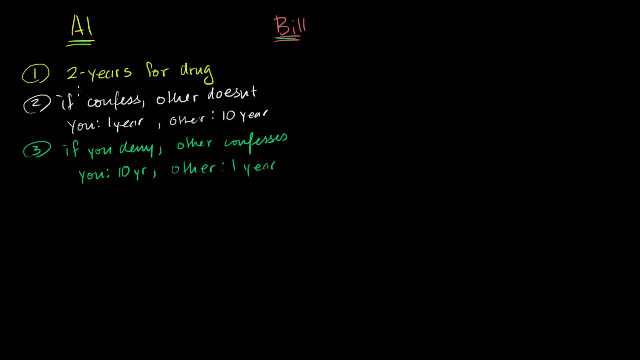 will get a reduced sentence, will get the one year. So this is like telling Al: look, if you deny that you were the armed robber and Bill snitches you out, then you're going to get 10 years in prison And Bill's only going to get one year in prison. 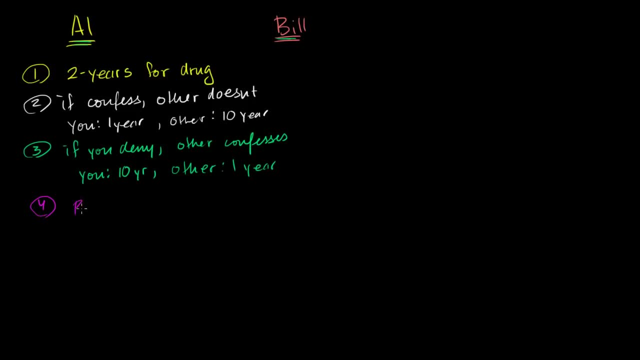 And if both of you essentially confess- both confess, you will both get three years. You will both get three years. So this scenario is called the prisoner's dilemma, Because we'll see in a second there is a globally optimal scenario for them. 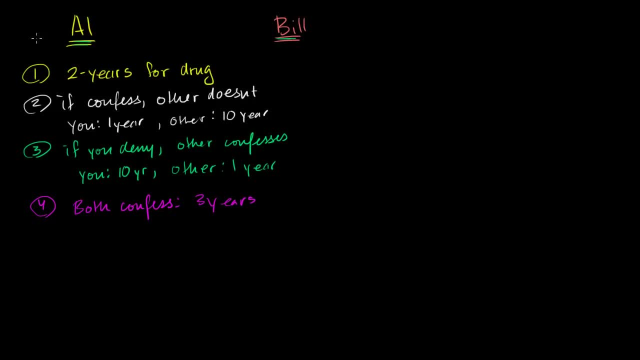 where they both deny and they'll both get two years. But we'll see- based on their incentives, assuming they don't have any unusual loyalty to each other- and these are hardened criminals here- They're not brothers or related to each other in any way. 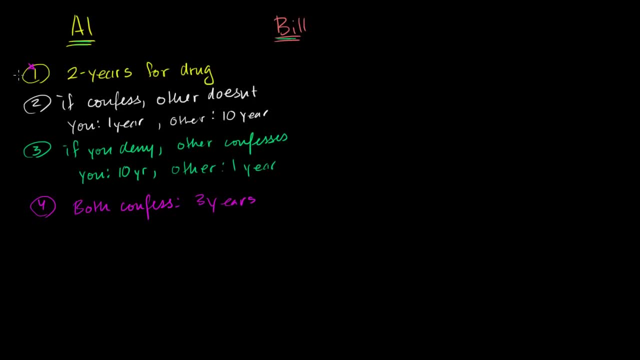 They don't have any kind of loyalty pact. We'll see that they will rationally pick a non-loyalty, Or they might rationally pick a non-optimal scenario And to understand that I'm going to draw something called a payoff matrix. 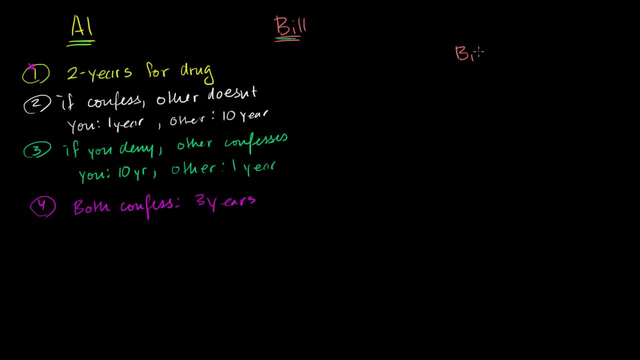 So let me do it right here for Bill. So Bill has two options: He can confess to the armed robbery or he can deny that he knows anything about the armed robbery. And Al has the same two options: Al can confess And Al can deny. 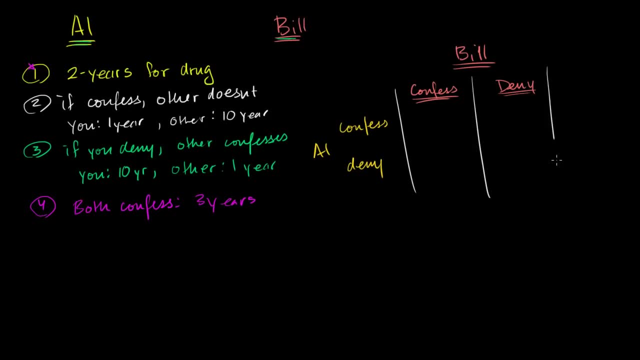 And since it's called a payoff matrix, let me draw some grids here And let's think about all of the different scenarios and what the payoffs would be. If Al confesses and Bill confesses, then we're in scenario four. They both get three years in jail. 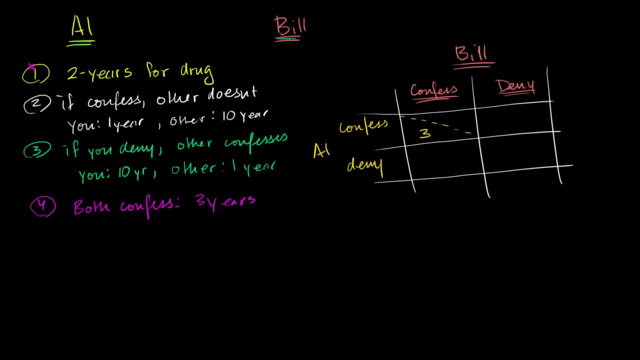 So they both will get three for Al and three for Bill. Now if Al confesses and Bill denies, then we are in scenario two from Al's point of view. Al's only going to get one year, But Bill is going to get 10 years. 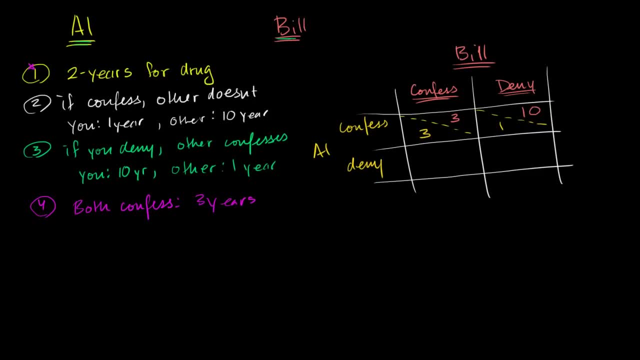 Now if the opposite thing happens- if Bill confesses and Al denies, then it goes the other way around: Al's going to get 10 years for not cooperating And Bill's going to have a reduced sentence of one year for cooperating. 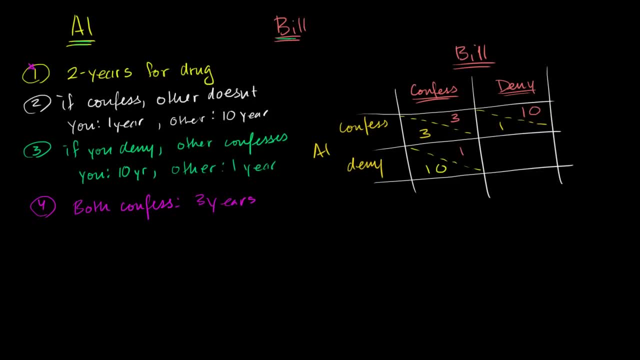 And then, if they both deny, they're in scenario one where they're both just going to get their time for the drug dealing. So Al will get two years and Bill will get two years. Now, I alluded to this earlier in the video. 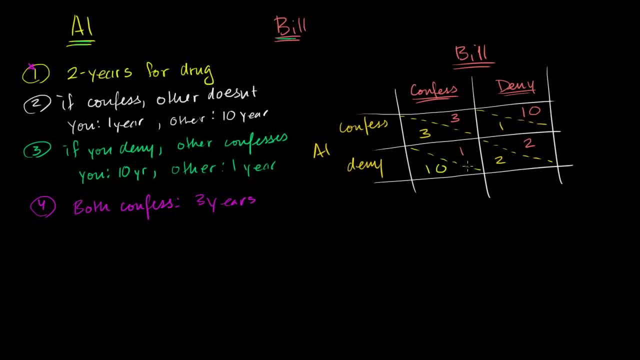 What is the globally optimal scenario for them? Well, it's this scenario where they both deny having anything to do with the armed robbery. Then they both get two years. But what we'll see is that it's actually somewhat rational, assuming that they don't have any strong loyalties. 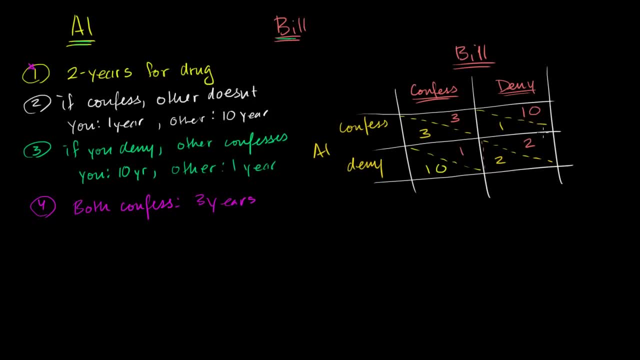 to each other a strong level of trust with the other party to not go there, And it's actually rational for both of them to confess. And a confession is actually a Nash equilibrium And we'll talk more about this. But a Nash equilibrium is where each party 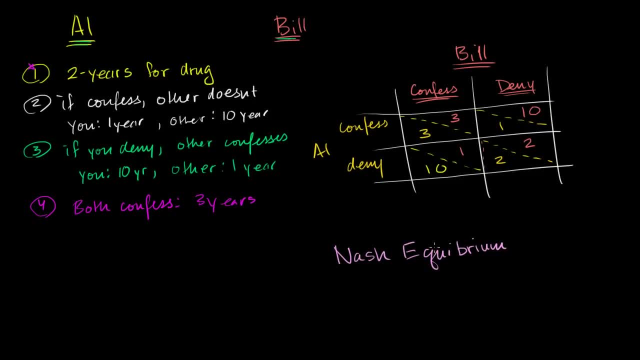 has picked a choice given the choices of the other party, Or each party has picked the optimal choice, given the choices of the other, or given whatever choice the other party picks. And so from Al's point of view, he says: well look, 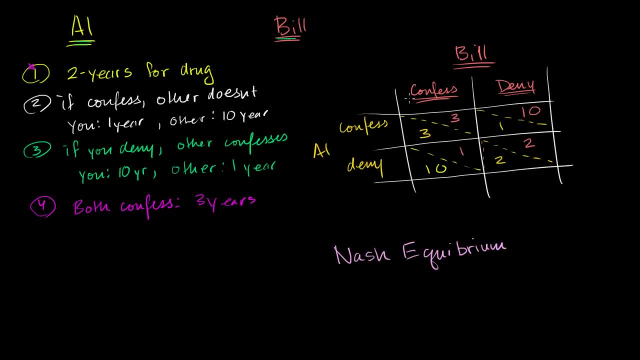 I don't know whether Bill is confessing or denying, So let's say he confesses. What's better for me to do? If he confesses and I confess, then I get three years. If he confesses and I deny, I get 10 years. 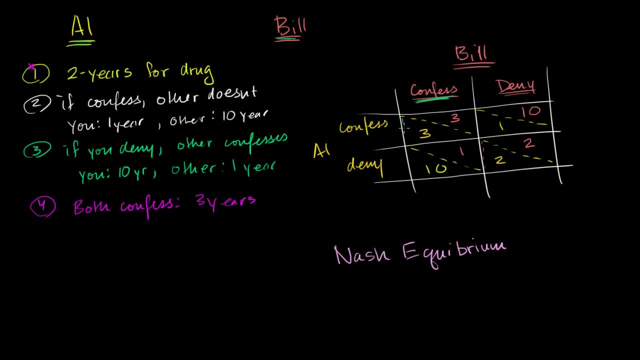 So if he confesses, it's better for me to confess as well. So this is a preferable scenario to this one down here Now. I don't know that Bill confessed. He might deny, If I assume Bill denied, is it true? 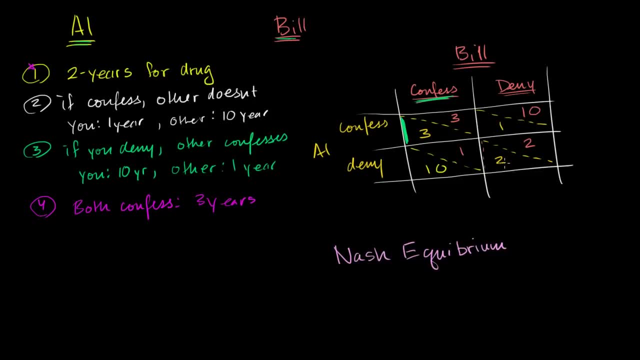 No. Is it better for me to confess and get one year, or deny and get two years? Well, once again, it's better for me to confess And so, regardless of whether Bill confesses or denies, so this, once again, the optimal choice for Al. 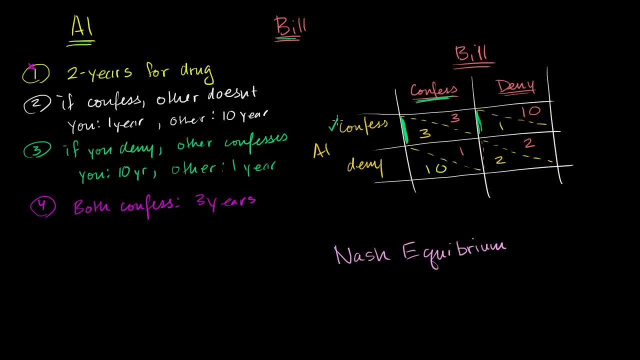 to pick, taking into account Bill's choices, is to confess. If Bill confesses, Al's better off confessing. If Bill denies, Al's better off confessing. Now we look at it from Bill's point of view And it's completely symmetric. 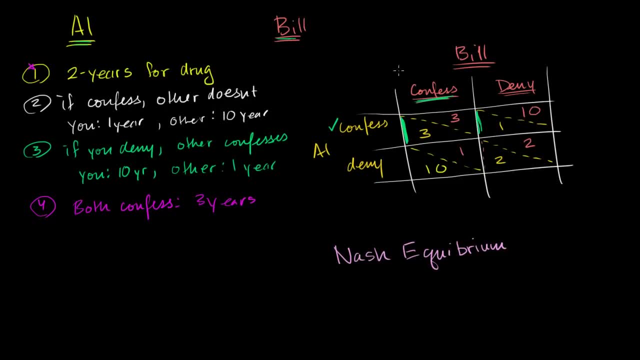 If Bill says: well, I don't know if Al is confessing or denying. if Al confesses, I can confess and get three years, or I can deny and get 10 years. Well, three years in prison is better than 10.. 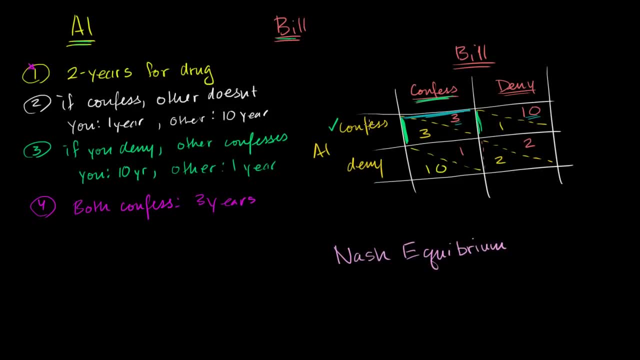 So I would go for the three years if I know Al is confessing, But I don't know that Al is definitely confessing. He might deny. If Al is denying, I could confess and get one year, or I could deny and get two years. 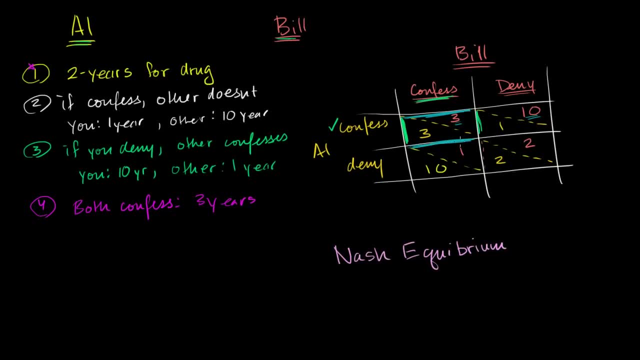 But once again, I would want to confess and get the one year. So, Bill, taking into account each of the scenarios that Al might take, it's always better for him to confess, And so this is interesting: They're rationally deducing that they. 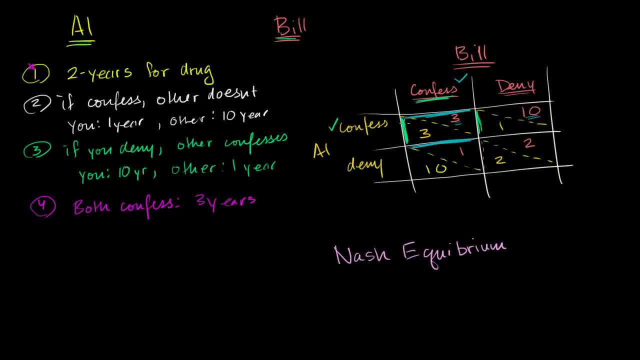 should get to this scenario, this Nash equilibrium state as opposed to this globally optimal state. They're both getting three years by both confessing, as opposed to both of them getting two years by both denying. The problem with this one is: this is an unstable state. 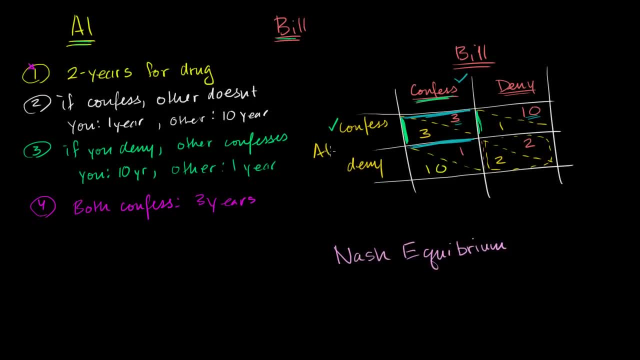 If one of them assumes that the other one has, If one of them assumes that they're somehow in that state temporarily, they say: well, I can always improve my scenario by changing what I want to do. If Al thought that Bill was definitely denying,